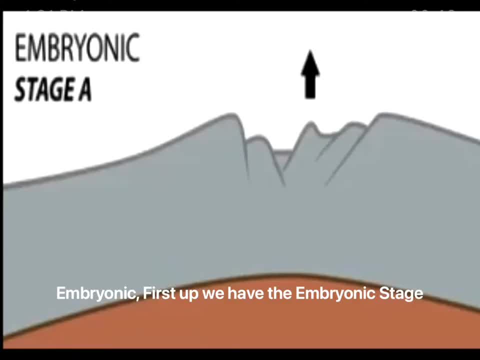 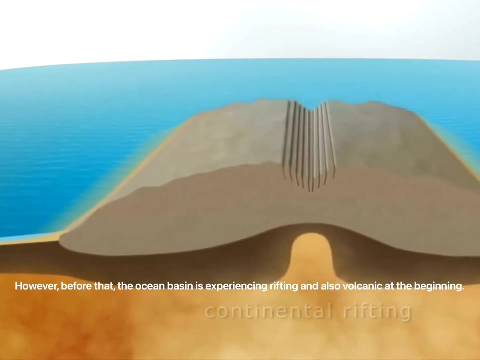 6 Major Stages of Ocean Basin Evolution. First up, we have the embryonic stage. Just like its name, embryonic is the first stage of ocean basin evolution. In this stage, the reef valley is formed while the continent begins to split. However, before that, the ocean basin experiencing rifting and also volcanic at the 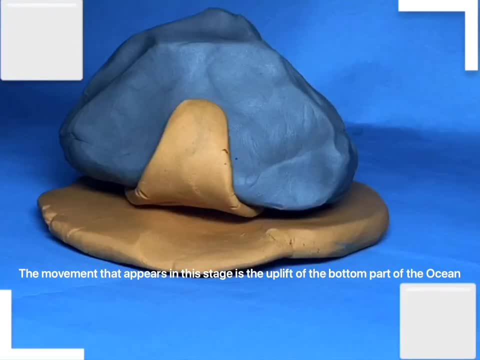 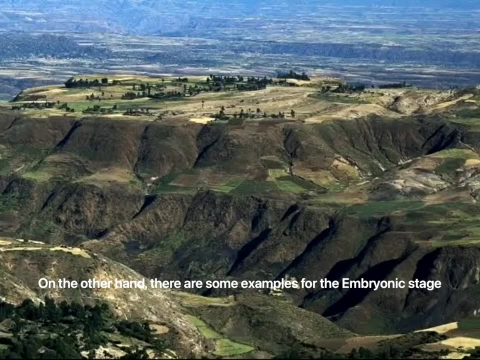 beginning. The movement that appears in this stage is the uplift of the bottom part of the ocean. This kind of movement allows the formation of reef valleys and the splitting of the continent. On the other hand, there are some examples for the embryonic stage, such as the Great Reef Valley. 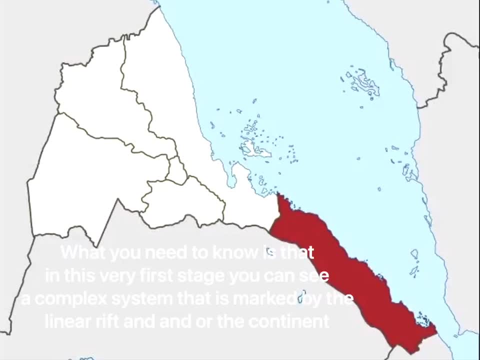 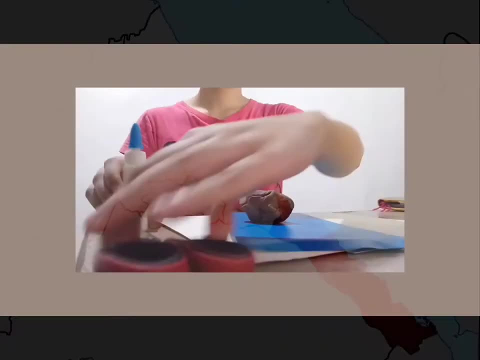 Southern Red Sea and Eastern Africa. What you need to know is that in this very first stage, you can see a complex system that is marked by the linear reef valley and or to the continent. After the embryonic stage, we have the juvenile stage. In this stage, 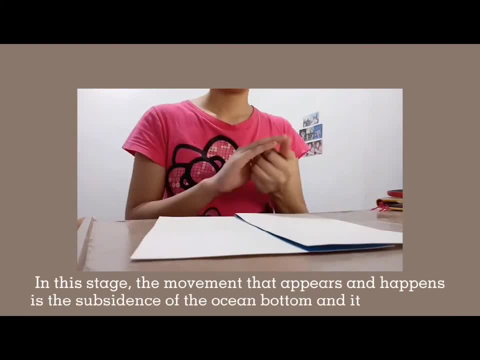 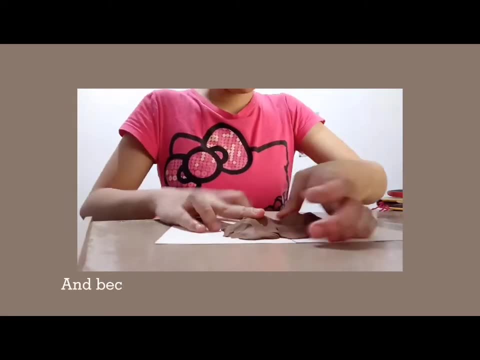 the movement that appears and happens is the subsidence of the ocean bottom and it will spread The subsidence and the spreading will create the divation of the continent And, because of this, the subsidence of the ocean bottom will create the divation of the continent. 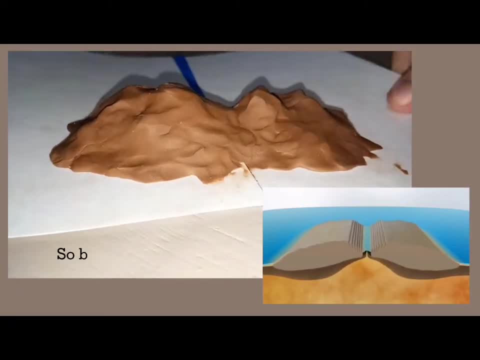 And because of this, the subsidence of the ocean bottom will create the divation of the continent. Because of the diverge, the seafloor basalt will be created. So, basically, when the separation happens, the gap is filled with the basalt, and that is how the basalt is created. 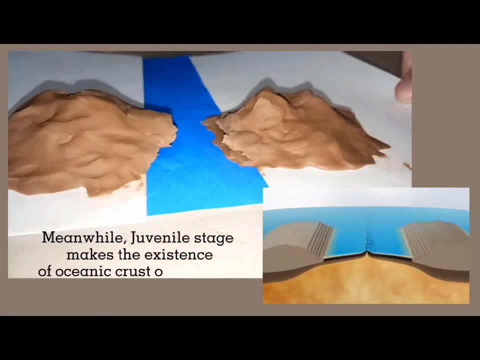 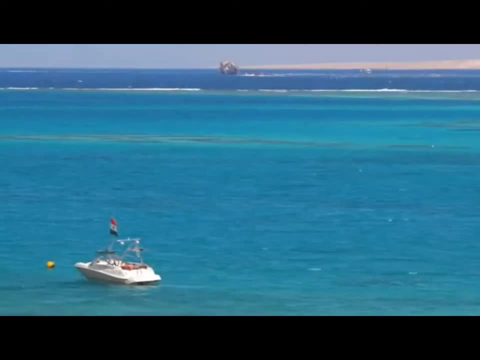 Meanwhile, juvenile stage makes. the existence of our shining crust occurs below the sea level with the shape of thin and dense. An example of juvenile stage is the Red Sea. In the Red Sea, a narrow deep axial zone is flunked on either side. 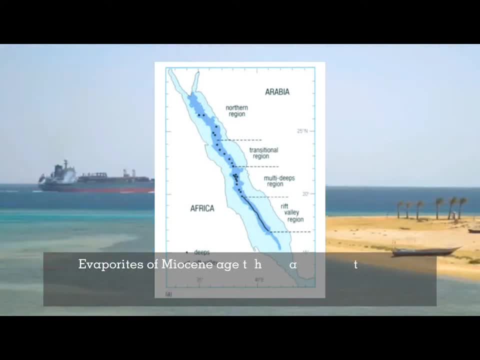 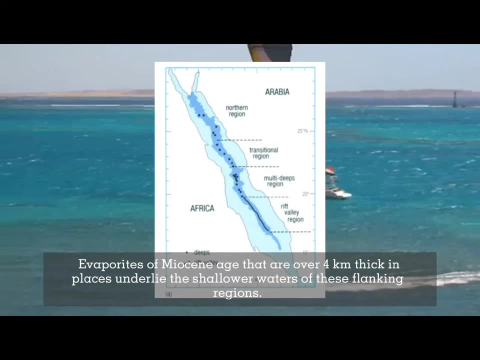 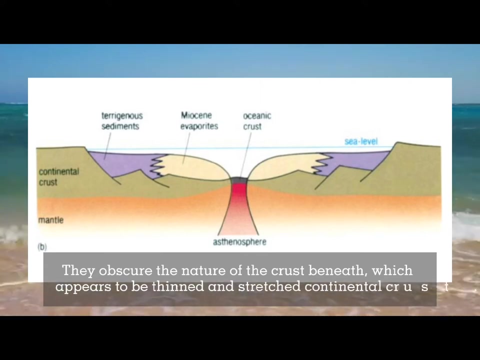 by a brush hollow area of a shelf sea. A vaporize of myosin H that are over 4 km thick on place underlie the shallower waters of these flunking regions. They obcurse the nature of the crust beneath, which appears to the tint and stretch continental crust. 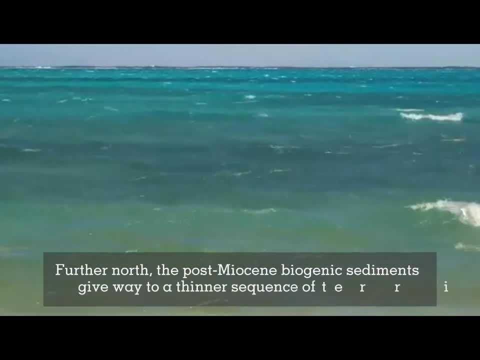 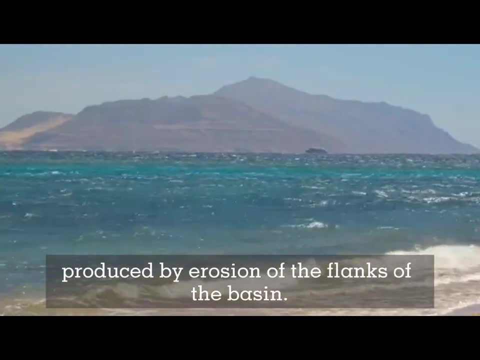 Further north, the post-myosin biogenic sediments give way to a thinner sequence of theriginous clays, suns and gravels produced by erosion of the plunks of the basin. Similar theriginous sediments can also be found interbed. 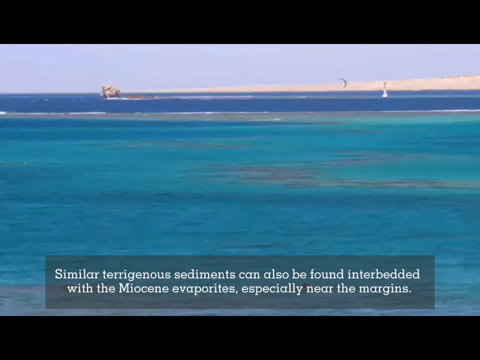 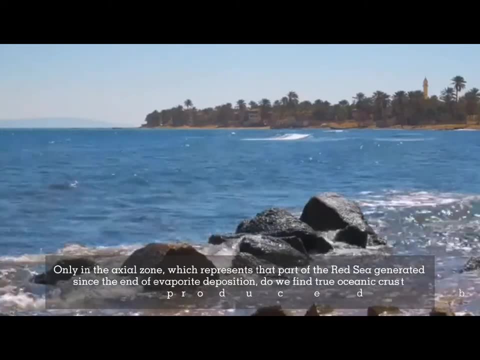 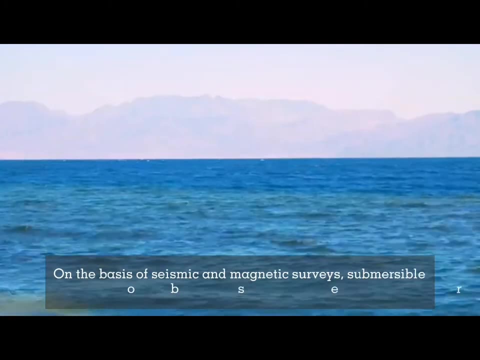 with the myosin and evaporites, especially near the margins. Only in the axial zone, which represents the depart of the Red Sea generated since the end of evaporite deposition, do we find true oceanic crust produced by sea floor spreading On the bases. seismic and magnetic surveys, submersible observations and sites, con sonar mapping. 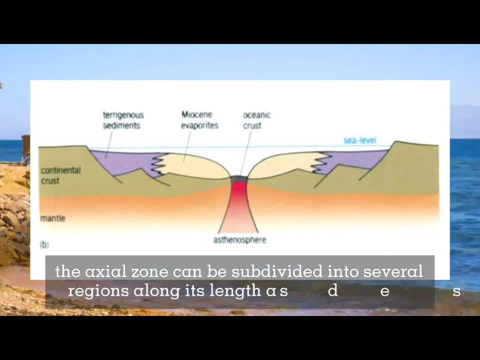 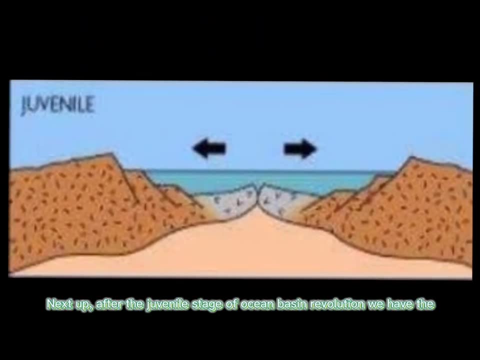 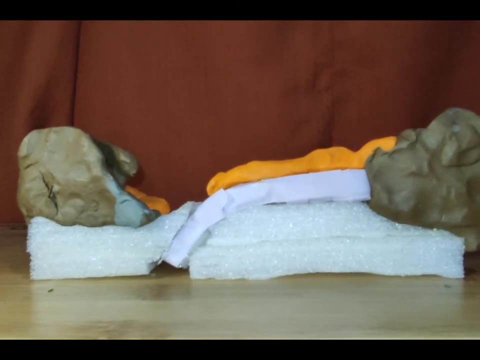 the axial zone can be subdivided into several regions along its length as described here. Mature: Next up after the juvenile stage of ocean basin evolution, we have the mature stage. For the mature stage, the ocean basin experiences widening, trench development and the start of subduction. 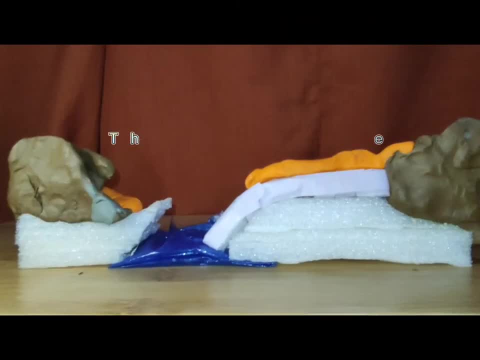 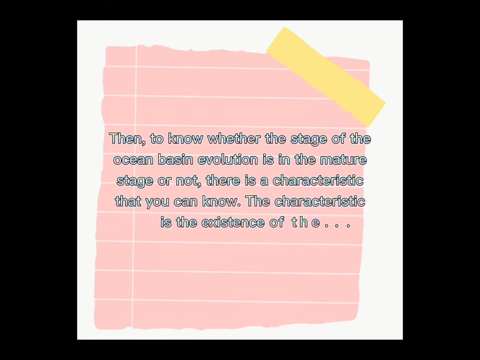 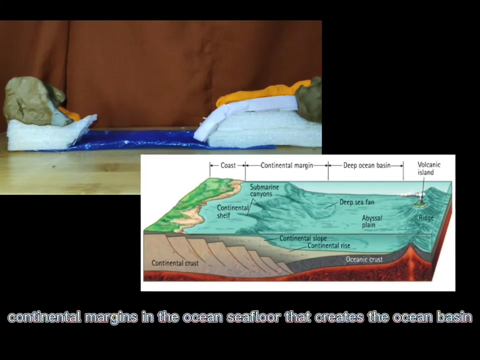 An example for the mature stage is the Atlantic Ocean. Then, to know whether the stage of the ocean basin evolution is in the mature stage or not, there is a characteristic that you can know. The characteristic is the existence of the continental margins in the ocean sea floor. that creates the ocean basin. 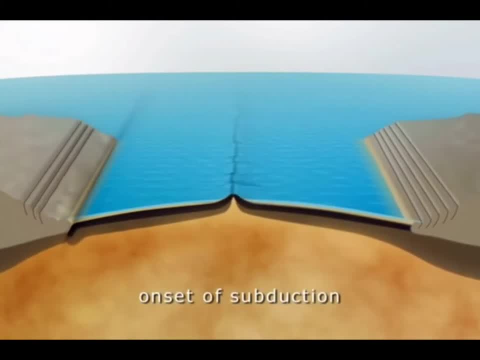 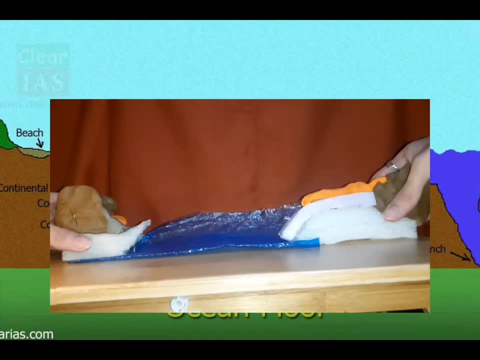 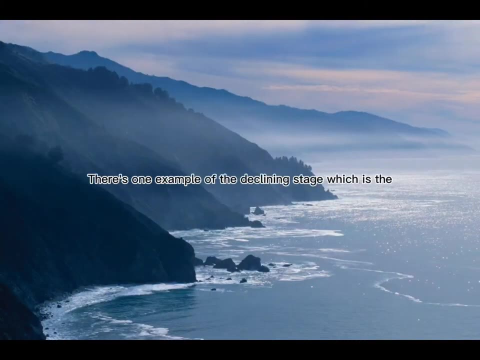 Declining Stage. Declining In the declining stage, the movement that appears and happens is the continuance of the subduction And because of this the ocean sea floor and also the ocean ridge is being eliminated. There is one example of the declining stage, which is the Pacific Ocean. 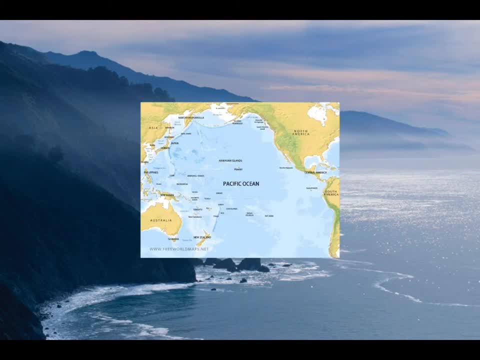 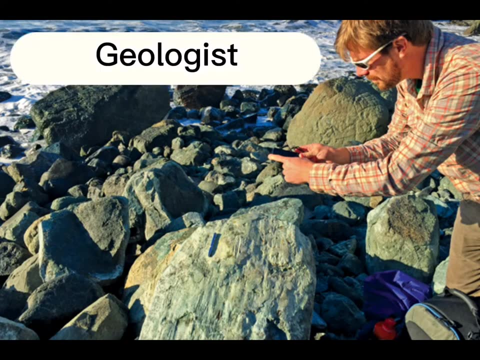 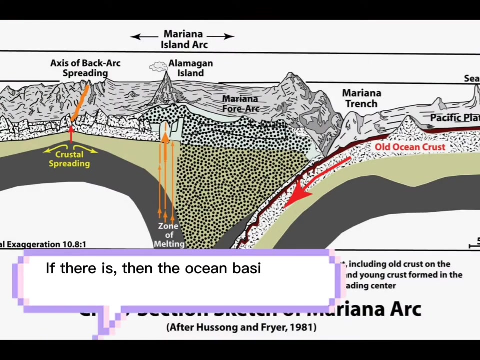 To know whether the ocean basin is in the declining stage or not. there is a character that differentiate this stage from other stages. In addition, usually the geologists will see whether there are island arcs and the island trenches around the basin edge or not. If there is, 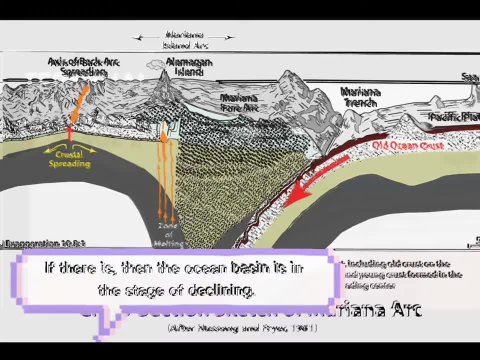 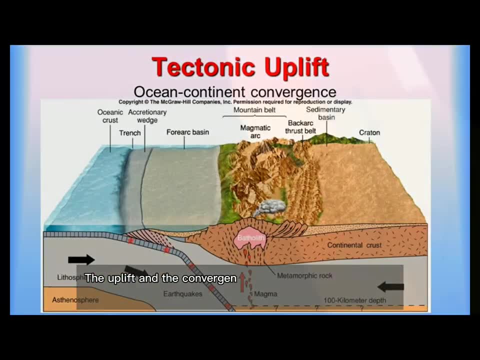 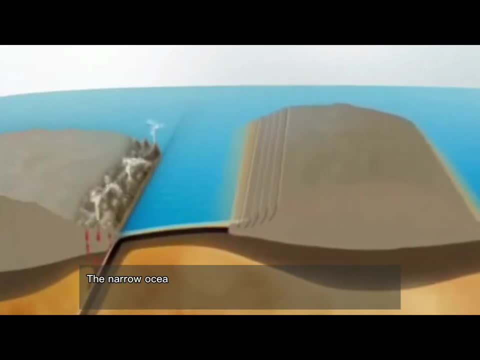 then the ocean basin is in the stage of declining. In the terminal stage, the movement that appears and happens are the uplift and the converge. The uplift and the convergence that is experienced by the ocean basin, creating the ocean basin, become normal. The narrow ocean basin may be caused by sediment input that makes the Yang Mountain exist. 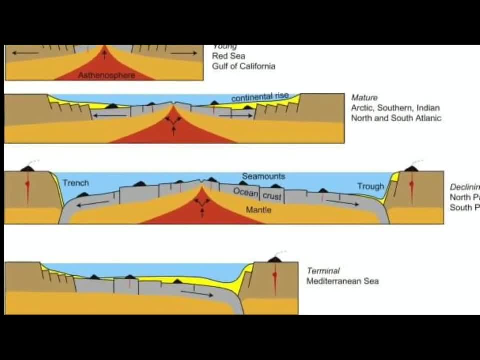 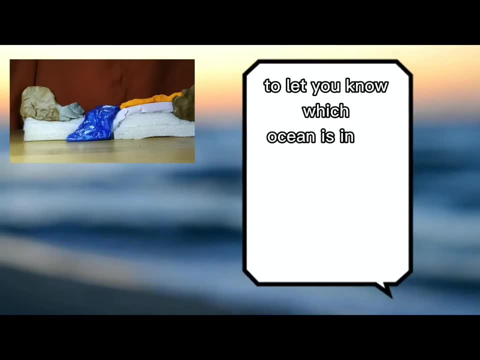 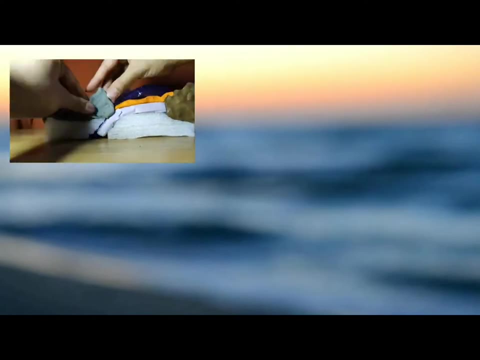 along and around the planks And in the terminal stage, the ocean basin that has been created is shallow. Meanwhile, to let you know which ocean is in the terminal stage or not, you can see the existence of the Yang Mountains in the ocean. If the ocean or the seas are narrow, irregular,